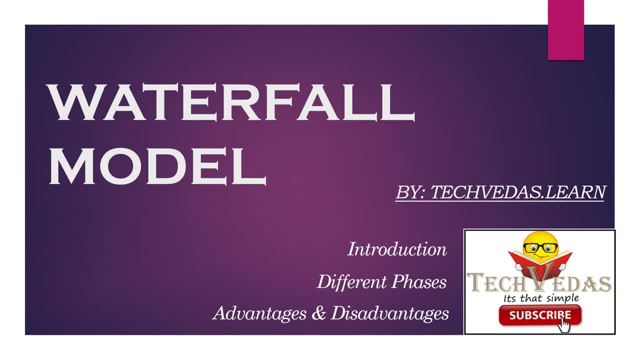 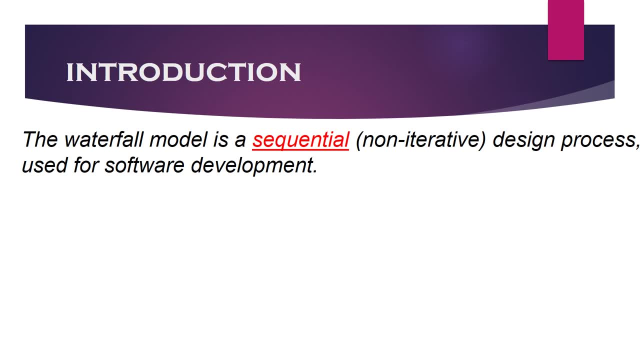 phases and some of the advantages and disadvantages of this model. So let's begin with the introduction of Waterfall Model. It's a linear or sequential design process for software development Means. there will not be any iteration possible during the execution of Waterfall Model. 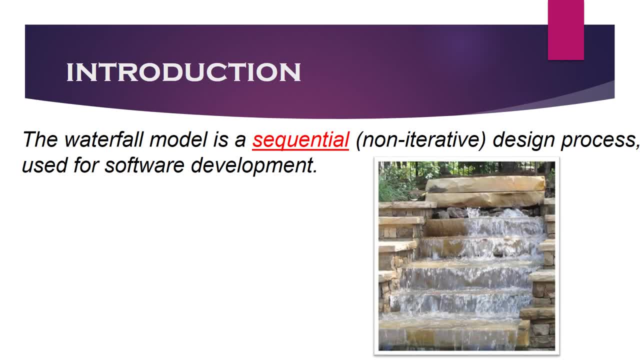 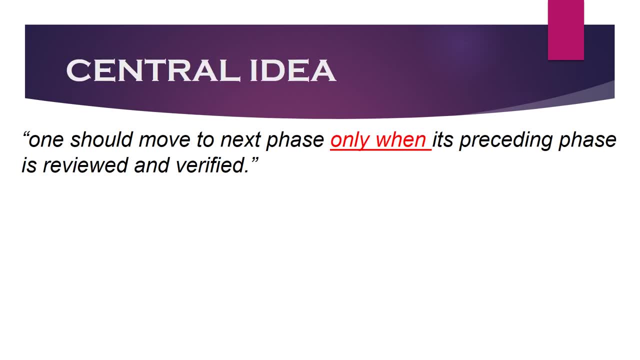 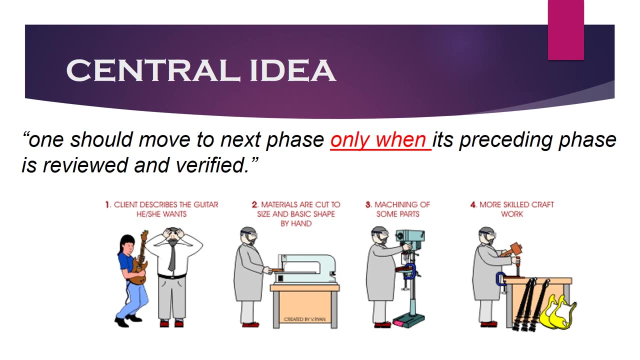 And this approach is largely one-directional: downwards, like a waterfall. The central idea behind this model is one should move to next phase only when its preceding phase is completed, And this is quite obvious, also as Waterfall is one of the oldest model, which was actually 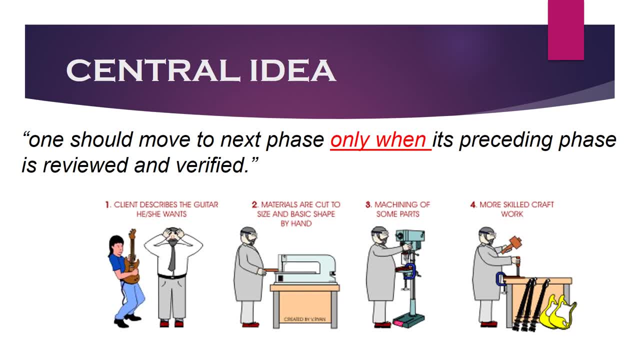 originated in manufacturing and construction industry, Where small changes also happen, Also become expensive much sooner as the development process starts. So in those days there was no formal software development methodology exist. Hence the hardware oriented model was simply adopted for software development. Waterfall model executes in the similar way, step by step, as the manufacturing of a guitar. 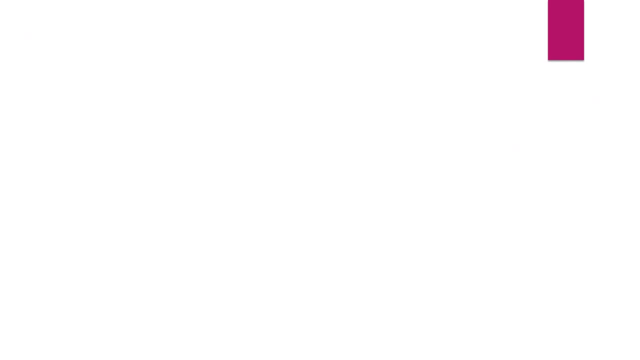 shown in the below picture. Now let's start. Let's try to look into different phases of Waterfall Model. It starts with the requirement phase, Where all the requirements will be collected from customer. Here requirements are set of functionality. what software should perform? 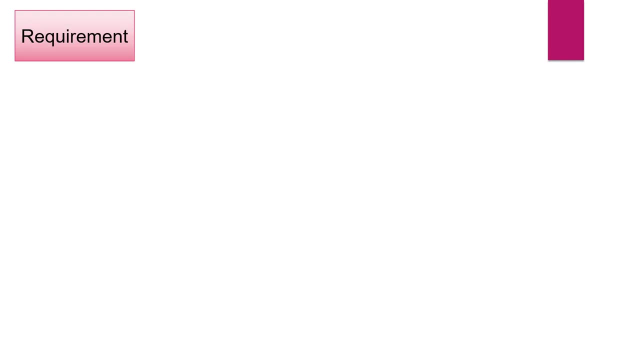 So once all the requirements are collected and documented, we move to analysis phase. In analysis phase, Subtopics requirements are broken down into subtopics and feasibility study will be conducted. The phase also contains time and cost estimation. So the whole idea of analysis phase is to make sure all the requirements can be implemented. 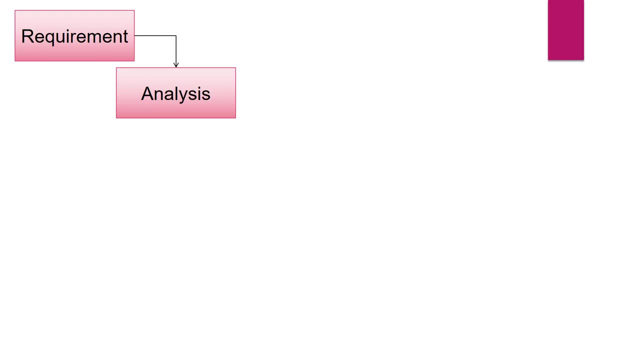 within the time and budget. And once the analysis phase is done, we move to the design phase. In design phase, software architect will draw the blueprint of the software which contains all the component which are need to be implemented. So at this step all the requirements are translated into their technical details. 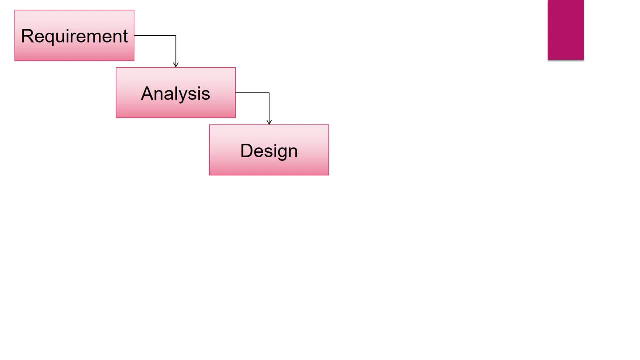 And finally results into two important documents: Low level design and high level design. Now, what is the design phase? Once the software blueprint is ready, we move to the coding phase. In coding phase, the actual software construction starts and white box testing is conducted. 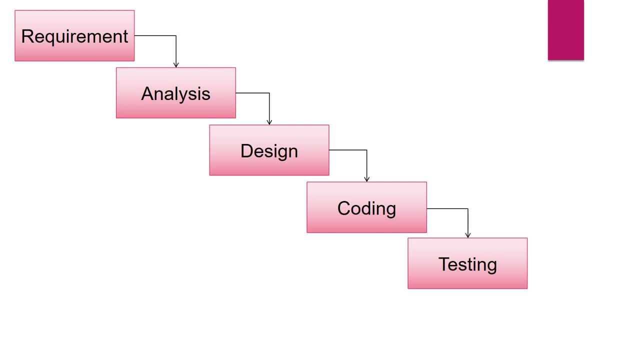 by the software developer. So once coding for entire software is done, we move to the testing phase, Where system test engineer validates the software against the requirements. So in this stage we move to the coding phase Here, once the software blueprints are ready, we move to the coding phase. 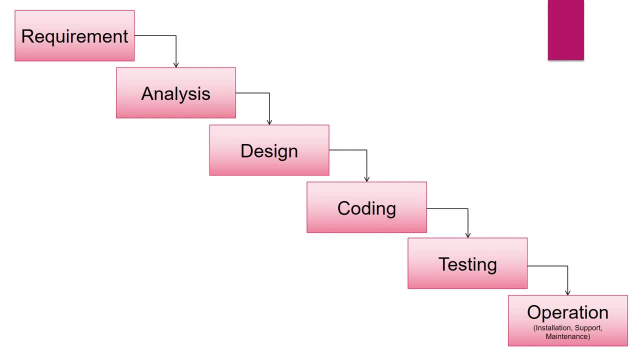 In coding phase. the actual software construction starts After completion of software testing. now we move to operation phase, where the software installation is done and required support and maintenance will be provided In operation phase. if there are any bugs or new requirements, we move to backwards altogether. 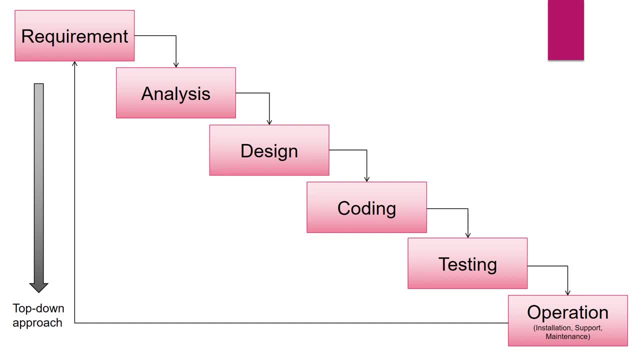 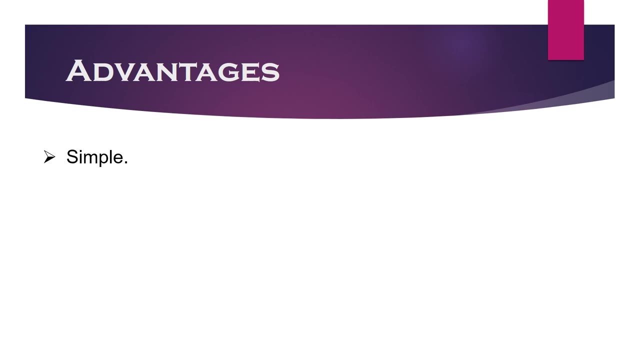 This is called as pure waterfall model. but to avoid rigidness of pure waterfall model, many modified waterfall model have been introduced like this one, which provides flexibility to certain extent. So after understanding different phases, now let's try to look into some of the advantages of waterfall model. 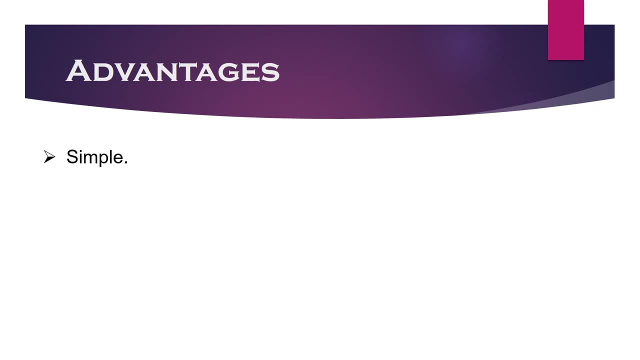 The first and foremost advantage of waterfall model is it's quite simple. Simple in terms of visualizing, Understanding and implementing. It also provides a structured way of doing things. It works well with the small projects where requirements are well understood beforehand and there are no technological hurdles. 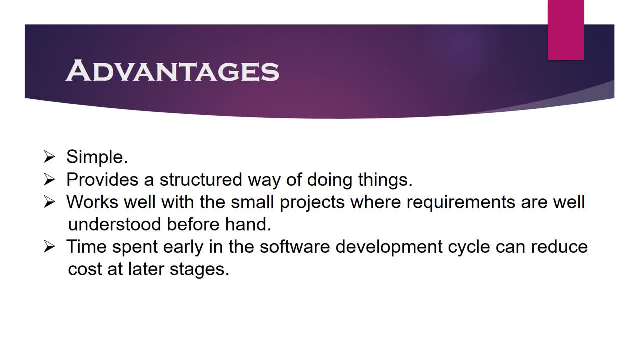 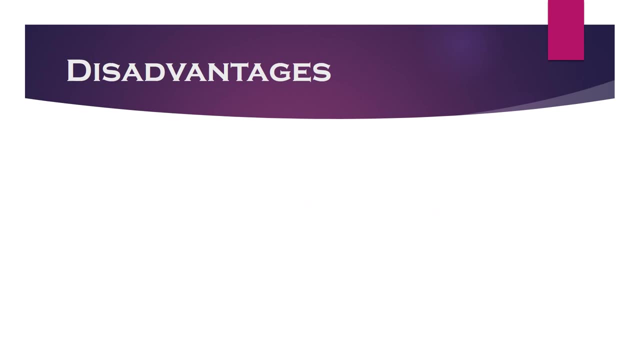 And at last waterfall model works with the philosophy that cost of finding bugs will increase. Waterfall model can move on in development phases So it emphasizes to spend good amount of time to understand requirement right from the beginning. Now let's try to look into some of the major disadvantages of waterfall model. 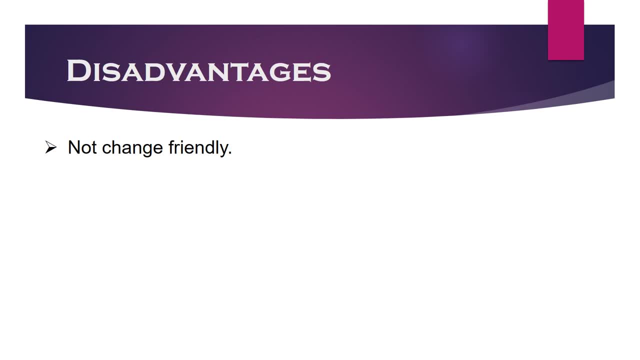 The biggest drawback of waterfall model is it is not change friendly Means. even though customer has realized an issue in requirement, Waterfall model resists to incorporate those changes in middle of the development. The other problem with this model is it's poor resource allocation. 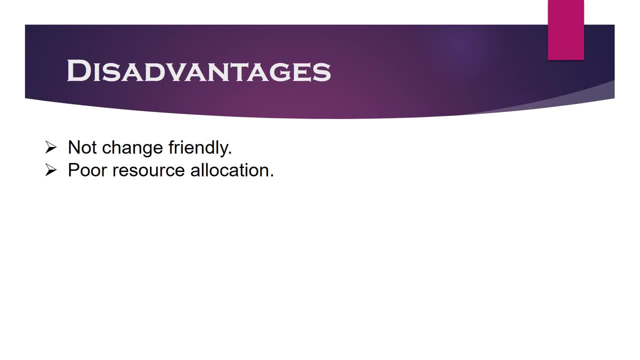 For example, a tester has to sit idle until the coding of entire software is completed. Also, a communication gap can result in completely different and unexpected output. The other problem with this model is It needs crystal clear requirements, But in many cases customer comes with very vague requirement. 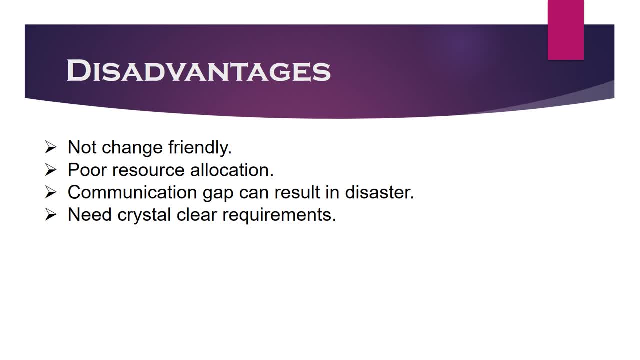 At beginning he might not be sure what in all functionality the software should perform. Until the end of all the phases, no working model of this software will be available for the customer to see the progress of the development And also It might be very difficult to foresee all the changes. 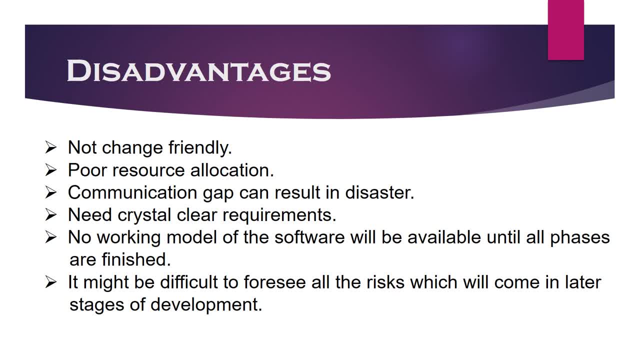 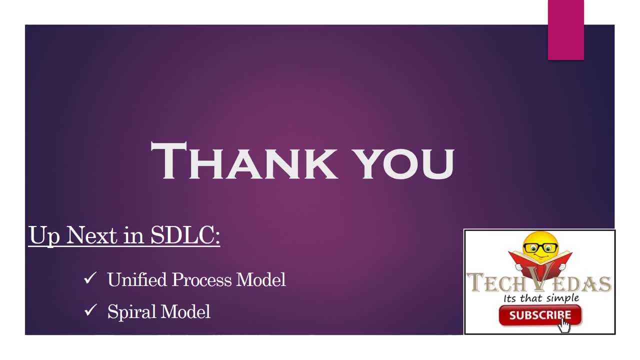 And also All the risk which will come in later stage of the development. So, friends, here we come to the end of this video. In summary, waterfall model is suitable for the projects where requirements are fixed and well understood beforehand And there are no technological hurdles. 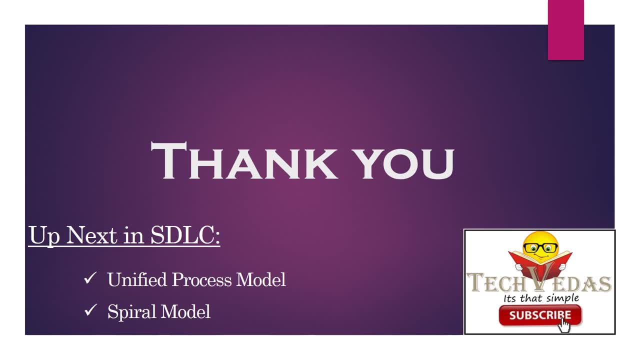 Please share your review on this video in the comment section and also subscribe my channel tech with us. dot learn For more videos like this, More future updates. Thanks for watching. Hope you like it.